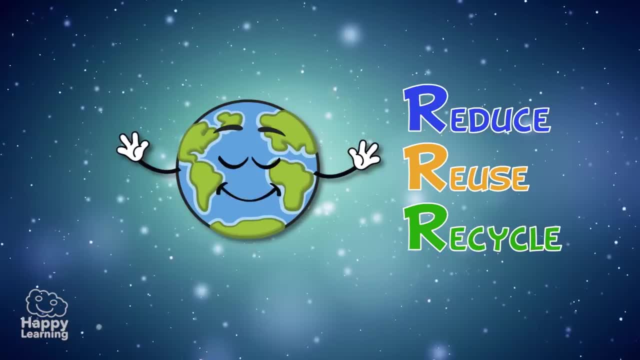 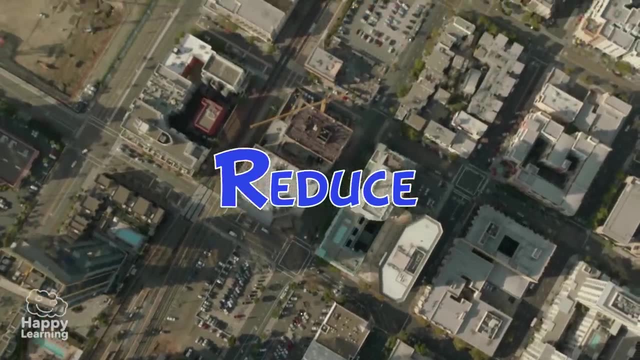 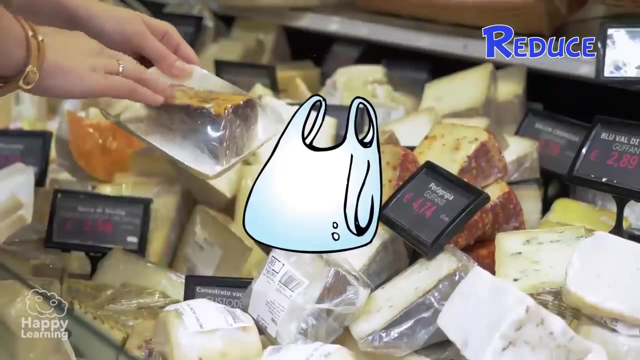 Those three words which can change the world. Do you want to know how? Yes, Well, let's find out. The first R is for reduce. If you think about it, there are many things you don't need. When you go to the supermarket, I am sure you can take your own canvas bags instead of using disposable ones given to you. 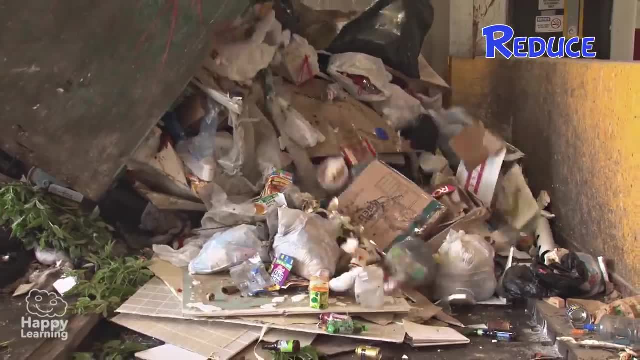 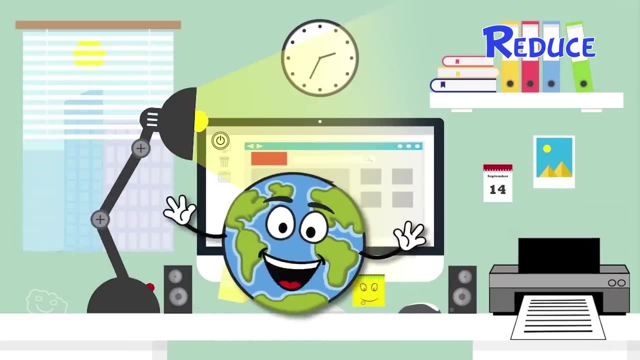 Like that, you will be reducing the amount of plastic, which is very contaminating, And I am sure that you don't need to print out so many documents or photos, nor leave lights, television or computers on when you are not using them. 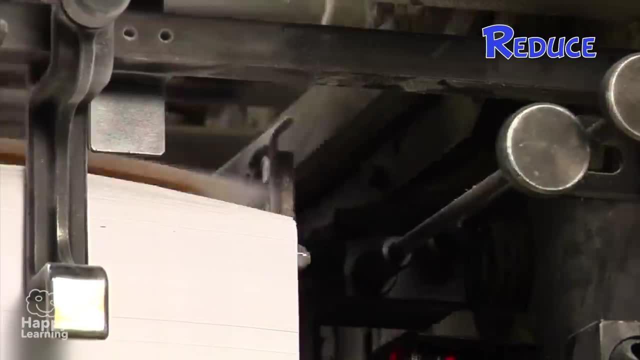 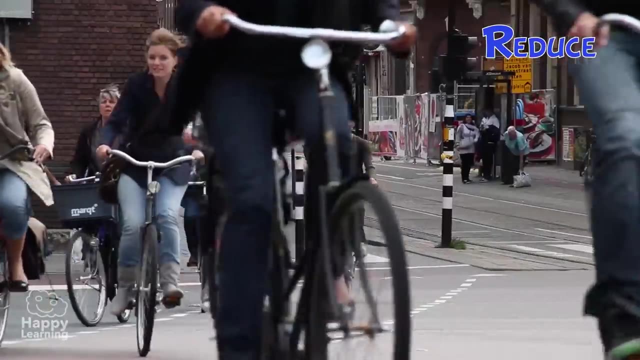 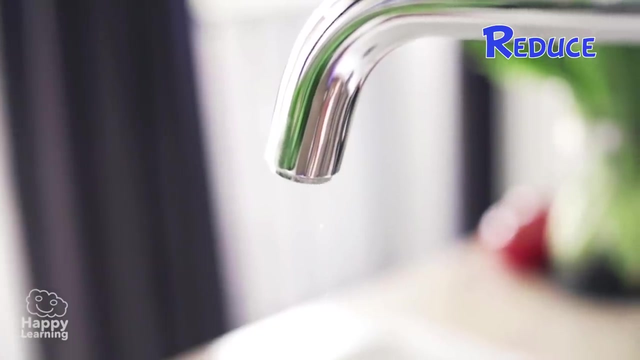 If you remember this, you will be reducing the amount of paper being used, as well as energy, and in turn, will be helping to reduce the contamination. And these are just a few examples. I am sure you can think of many more different ways to reduce what you are using or creating unnecessary waste. 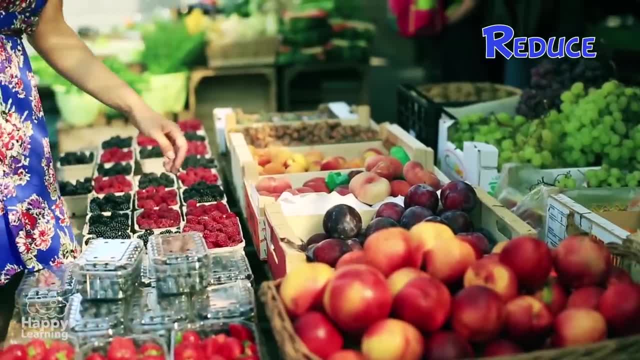 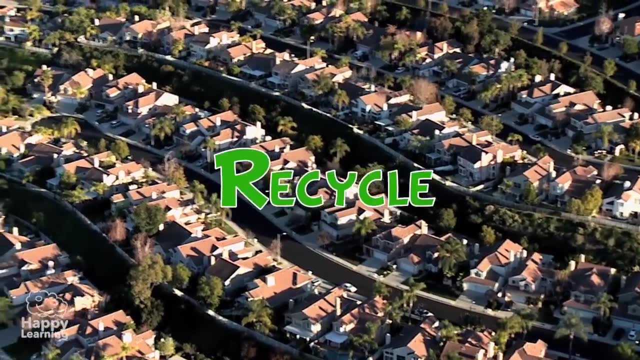 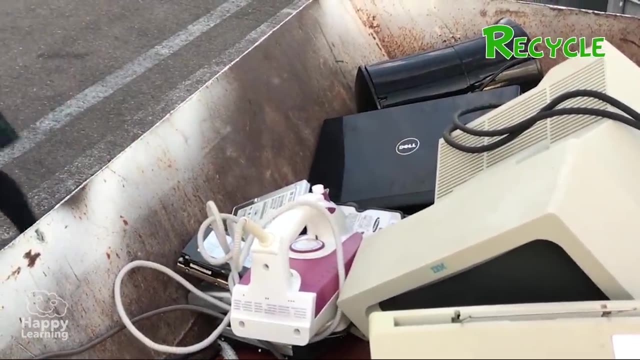 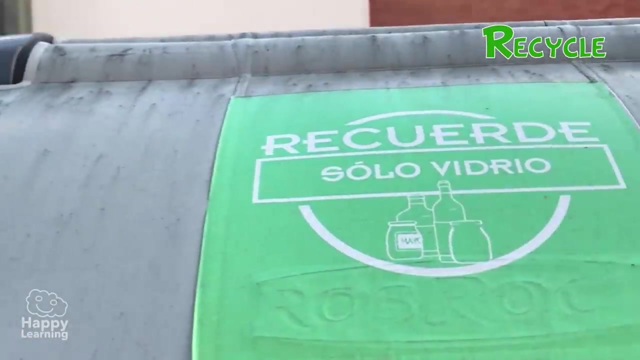 The following question will help you with this task: Do you really need this or is this just a whim? The second R is for recycling. Now it is easier than ever to recycle things we don't need anymore so that they can be reused. Near your home, you can find places like the recycling station and containers for cans, plastic, paper or organic waste. 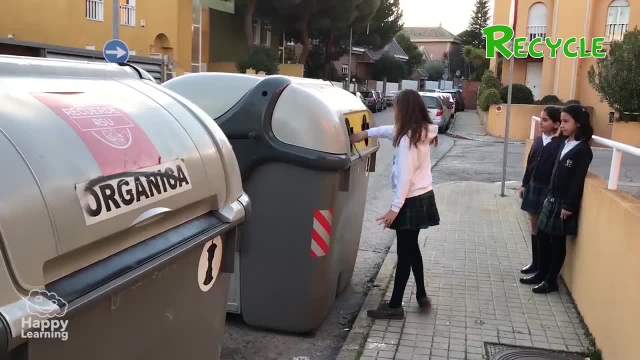 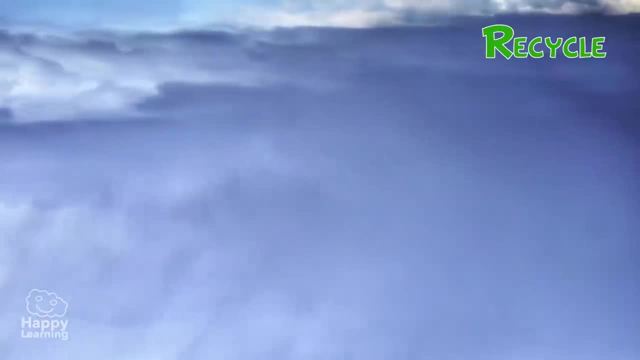 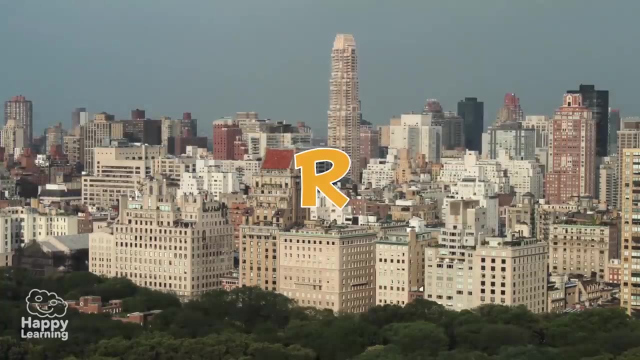 They each have specific colours to make it easier to identify. By using them, you will avoid contaminating nature, the rivers and seas, as well as the atmosphere, which is the air we breathe. And finally, we have the third R, which refers to reuse. 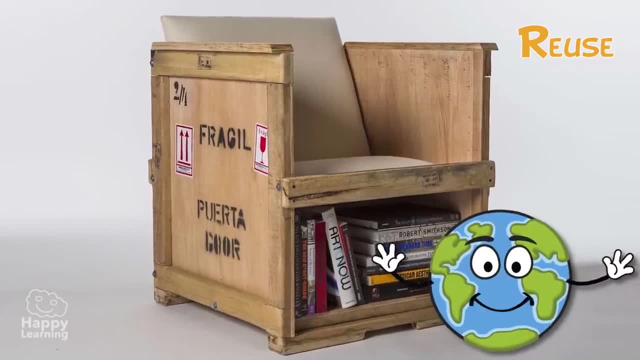 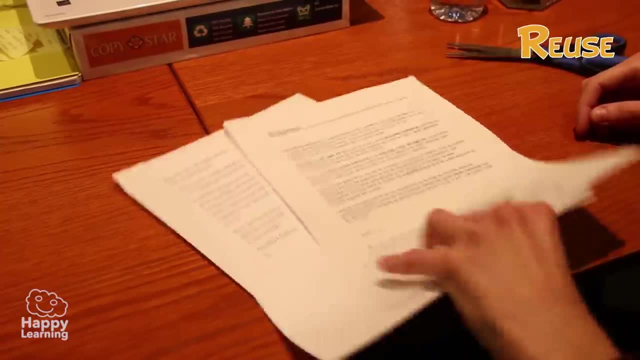 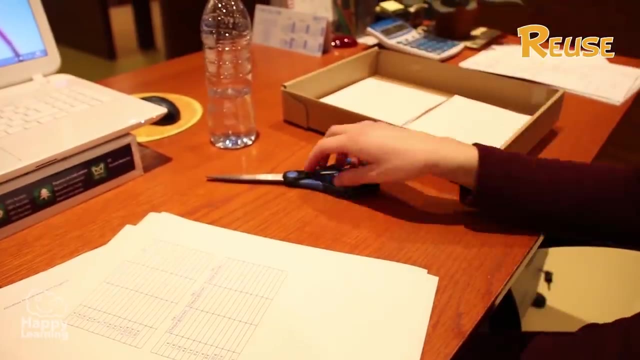 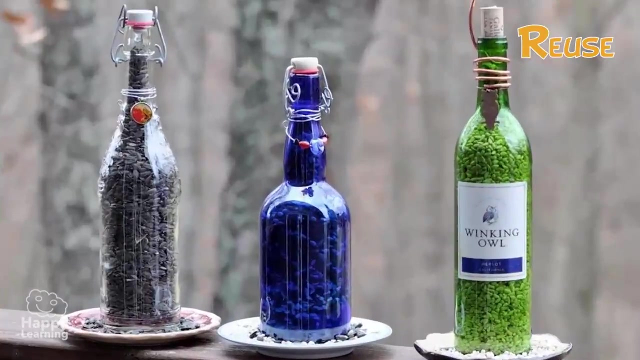 How many things do you think we can reuse again and again instead of throwing them away? Let's see A piece of paper that has only one side, One side printed on A carton box, A plastic bottle. You think now, With just a little bit of imagination, I am sure you can come up with many more exciting and fun new uses for them.